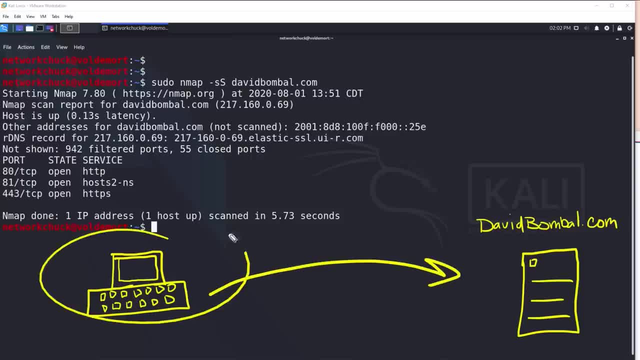 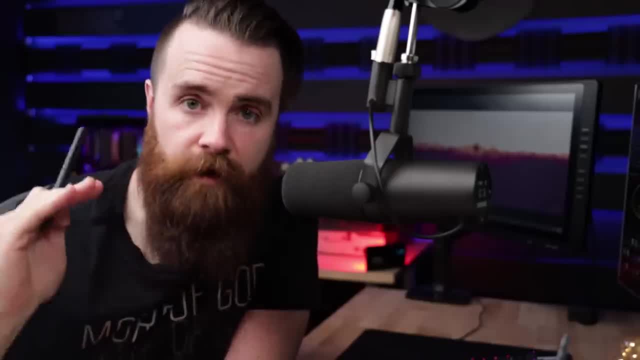 to hide the fact that all of these messages, all these attacks are coming from you. you're in trouble, or at least are very close to being in trouble. now, before i show you how to hide yourself, let me tell you this. i'm speaking strictly in the context of ethical hacking: having a business's 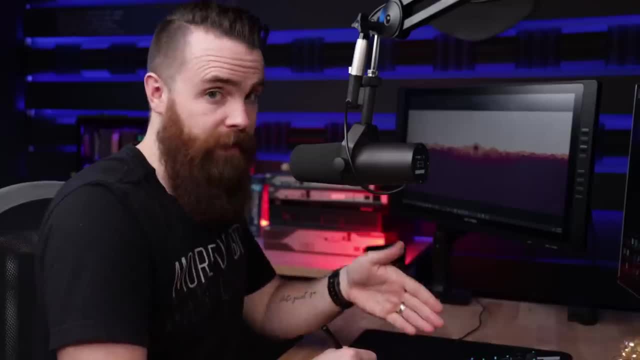 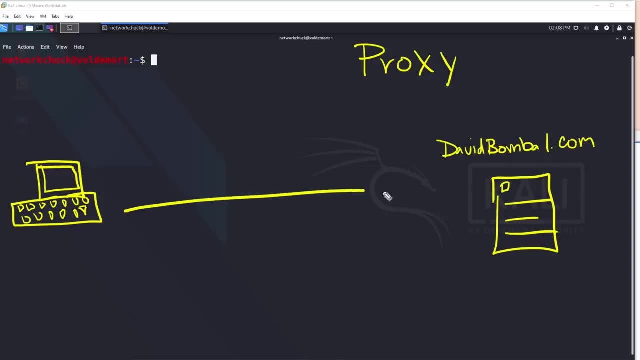 explicit permission to do this. anything else, don't do it. there are a few ways to hide yourself, but i want to focus on proxies and, more specifically, proxy chaining. how does that work with the proxy? instead of sending all of our attacks directly to david, from us telling david exactly who's doing it- hey, it's me- we'll use a middleman, a go-between. 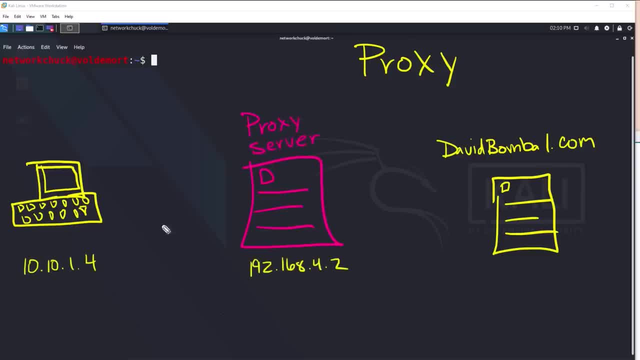 a proxy, we'll call these proxy servers. so now when we attack david, we'll send our attacks through the proxy server and if david does happen to catch on and see the attack and he goes, hey, who's attacking me? he'll see the ip address of the proxy server and not us. now we have to be careful here because 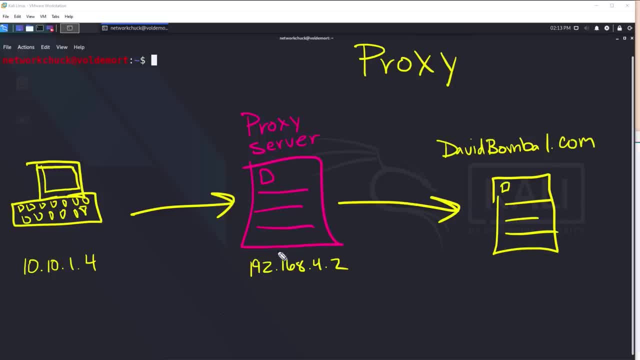 what could happen is david would tell the police: hey, someone's attacking me, and the police see the attack and we're gonna contact them and find out who attacked you. and the proxy server will have logs, logs that could tell them that, hey, it was actually this guy over here, you, that used the. 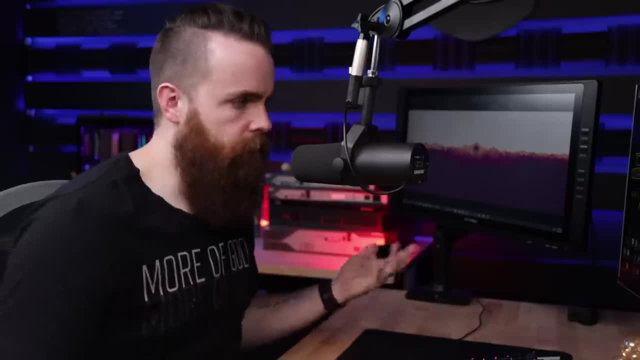 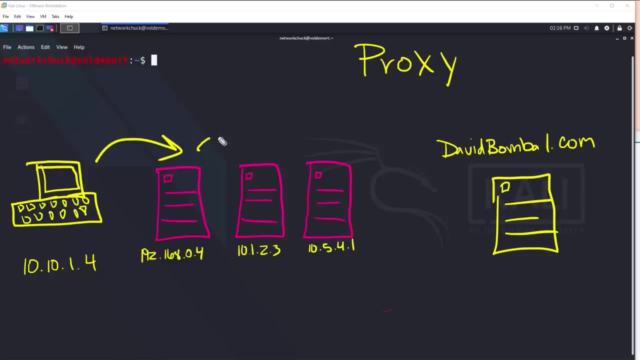 proxy server to attack david, and then you're busted. so what do we do? well, um, let's use some more proxy servers. how about that? instead of sending our attacks through just one proxy, we'll send it through multiple proxies. send it to this guy, then hop to this guy, then hop to this guy and 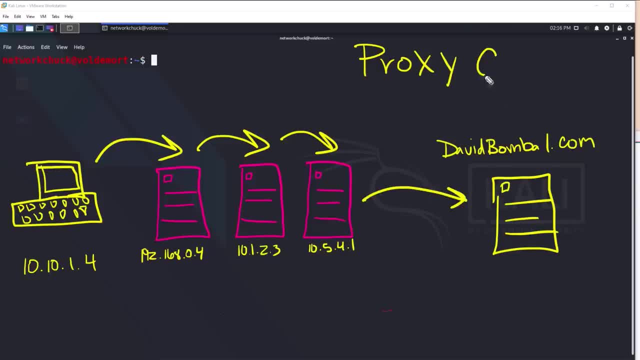 then, finally, we're attacking david. this is what's called proxy chaining: we're chaining together. so if david did tattle on us and tell the police the odds of them going through each of these servers and going through their logs and finding us through all this mess, pretty slim chance now. 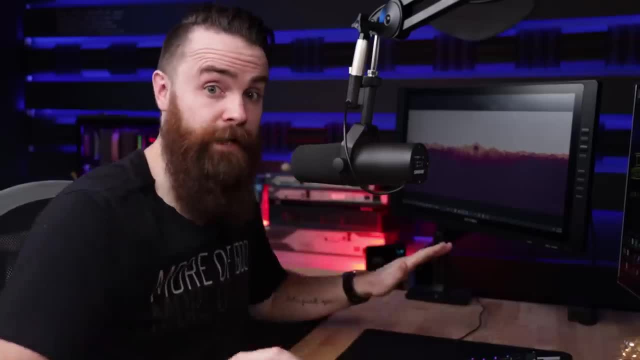 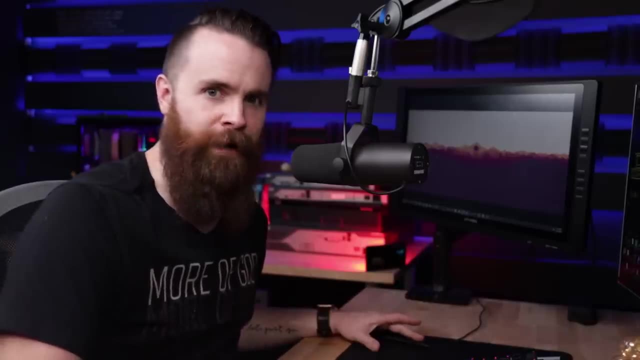 not impossible. this is not a foolproof situation where you'll never be discovered no solution is, but it does make it crazy difficult. so, uh, how do we do it? let's do it right now. we're going to use an app called proxy chains which, if using cali, should be pre-installed. all we have to do is 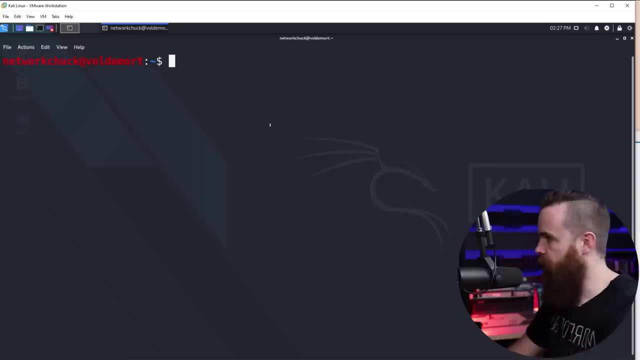 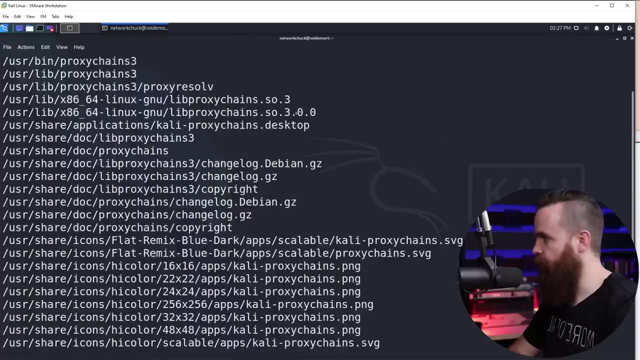 configure it. so first we gotta locate the configuration file. so here at the command line, and i'll type in proxy chains: hit that and the first option up there should be where your stuff is. yep, right there, etsy forward slash proxychainsconf. the reason we use this command is yours. 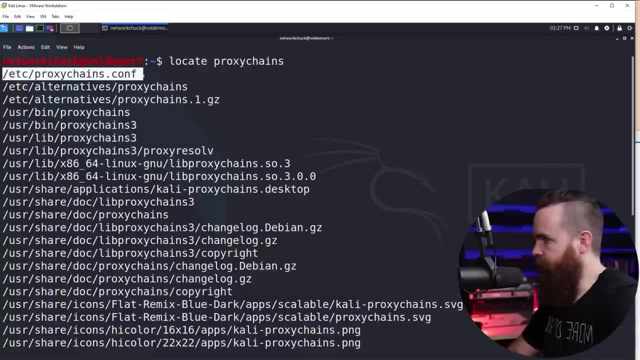 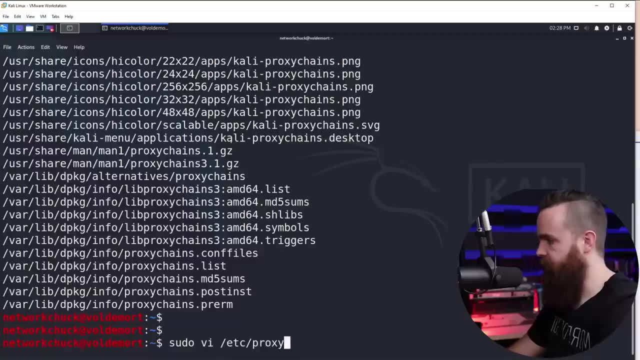 could be in a different spot. this will help you find it and this is the file we're going to edit. so i'm going to jump in there, i'll do sudo and i'll use vim as my editor. so i'll hit vi and then i'll put my path in etsy proxychainsconf. now there are three main modes we can run this in, and 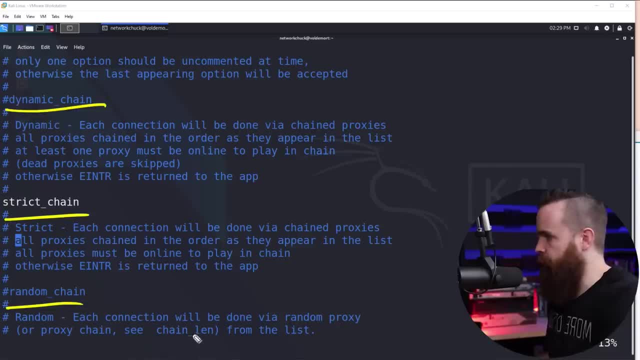 one we're going to ignore dynamic, dynamic, strict and random. we're not going to do strict, so we're actually going to end up commenting that out with a hashtag. with dynamic, we'll put our list of proxies in. we can have a lot. let's say we. 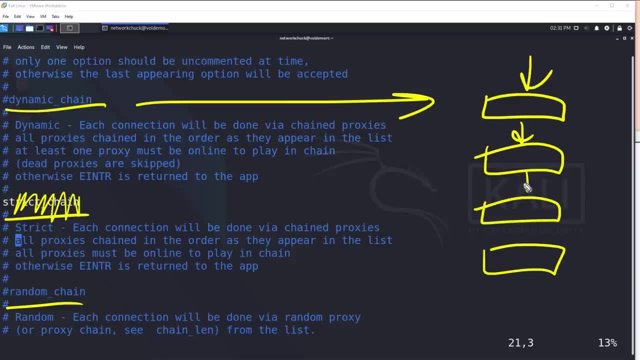 have four dynamic will go through each proxy in our list and chain them together and use it in the order we put them in every single time, unless one of them is out of commission, not responding, not usable, it'll just skip it. with random, it's um, it's random, same deal. let's say we have a list. 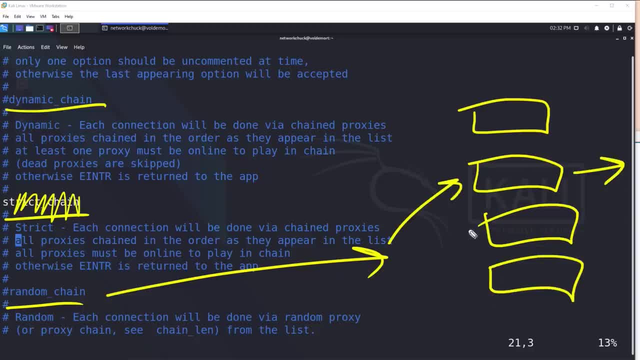 of four proxies. it will randomly choose one proxy to use, which is fine in a lot of cases because it your target's guessing like, oh, where's it coming from? where's it coming from all these different ip addresses? but personally i like dynamic because we put a lot of proxies in between us and the 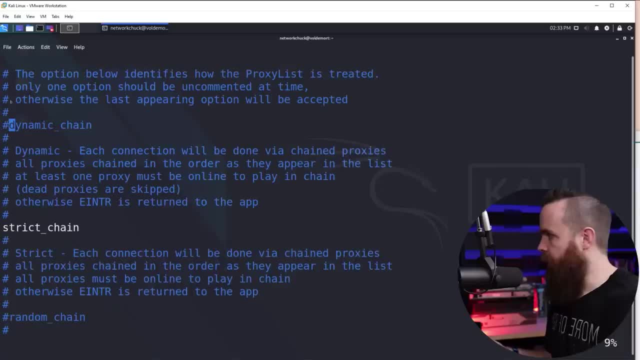 target, making it harder to find us. so to make that magic happen, i'll put my cursor there, i'll hit i for insert and i'll remove that hashtag which makes that configuration active. and we want to comment out or put a hashtag in front of strict chain disabling that option. so we got our mode. 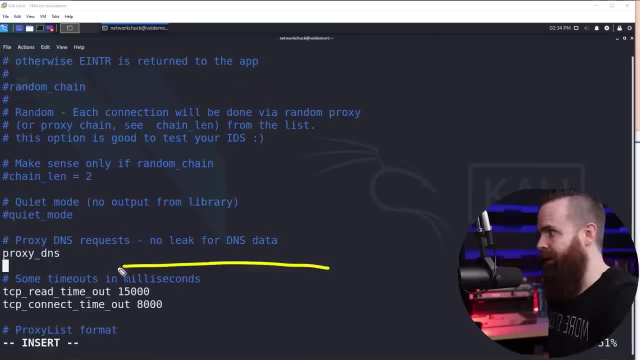 we're not done yet. let's keep going. we're going to scroll down. now. here's an option we're not going to touch, but it's good we have it enabled by default. proxy dns if we were to comment the setting out and not use it. our dns request. 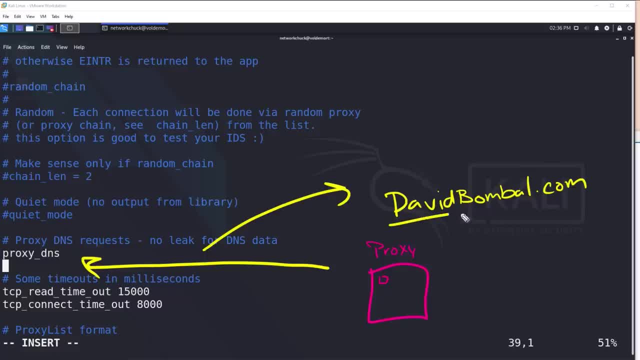 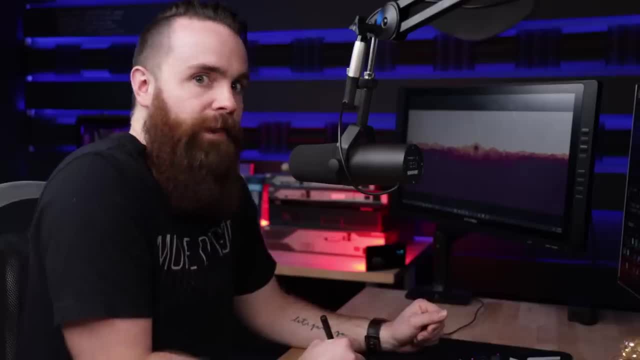 would still be coming from us. so when we try to discover what ip address davidbombacom has, that particular request would come from our ip address, let's just say 10.1.0.4, and that could be a way that people find out where the hacker. so best case is you want to proxy everything, even your dns. 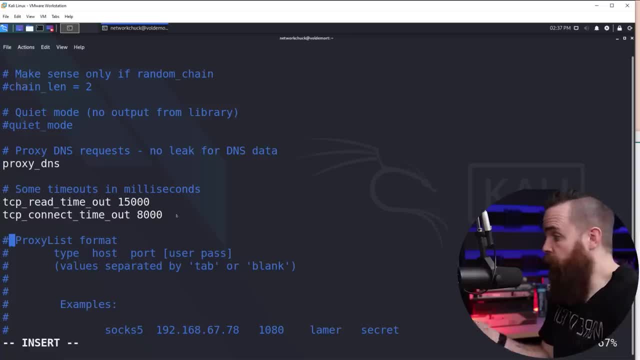 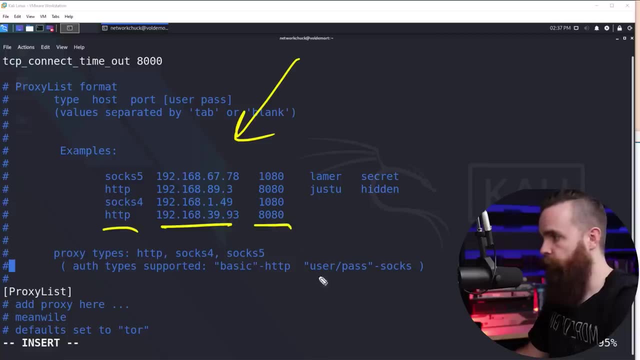 request through your proxy. that way, no one could find you now as we scroll down. the only thing we have to look at now is our list of proxy servers, and here's the format right. here we have the type, the server ip address and the port we're going to use, and if it has authentication, you'll put the username password. 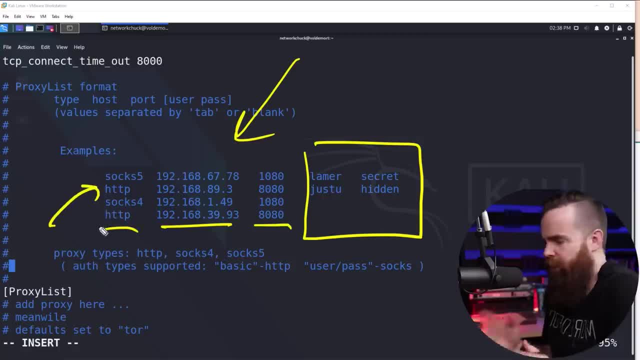 right here now. you might be wondering: what's with the different types? what's the difference? we're not going to cover that right now. it's a whole other video. just know that socks 5 is better than socks 4, as you might assume, and in addition to http, we also have https, so all you have to know. 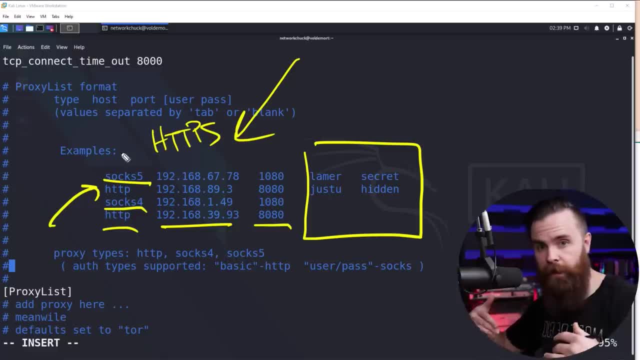 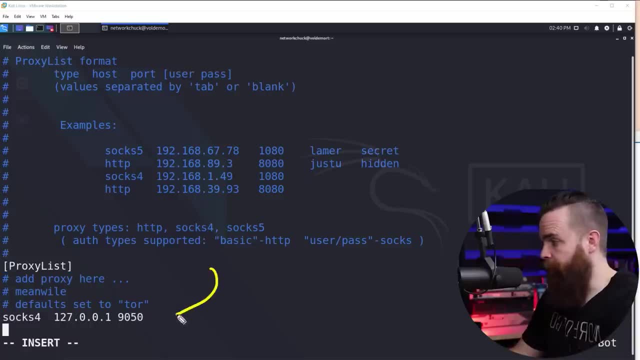 right now is. these types will help you proxy your connections, help you to hide yourself. some are more secure, like https or socks 5.. so let's move on past the example and start adding our list now. by default, we already have something here. this proxy server is pointing to 127001, which 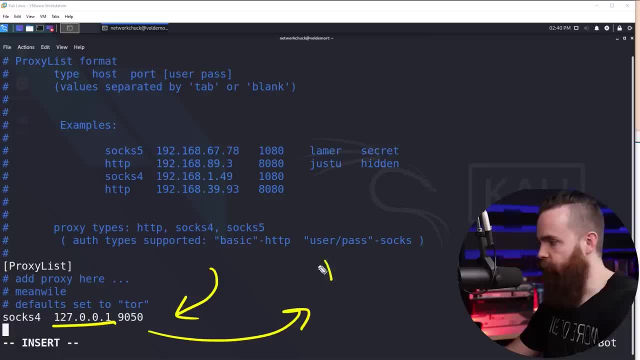 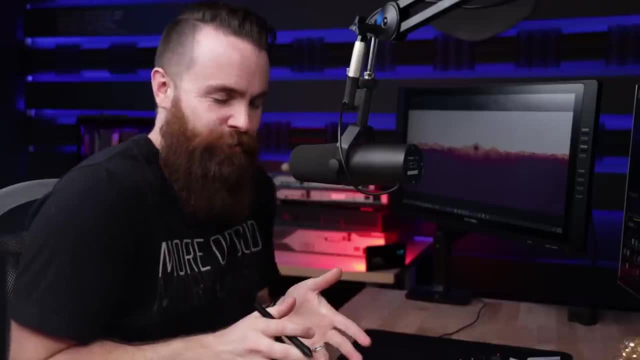 is just pointing to us. this default config is actually going to be using what's called tor or the onion router. we would have to have this service enabled on our kali linux box here. we're not going to mess with tor right now. just know, it's your gateway to the dark. 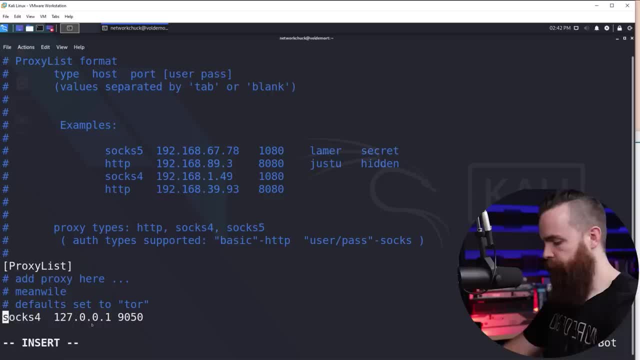 web and there's a lot of proxies involved, so we're going to skip that for now. so i'll put a hashtag in front of that to comment that out and i'm going to put my first server in the type of this proxy will be socks 4 and then i'll put a space between that and the host ip address and then a space. 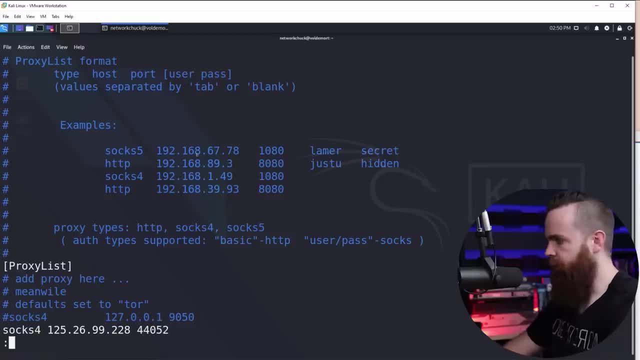 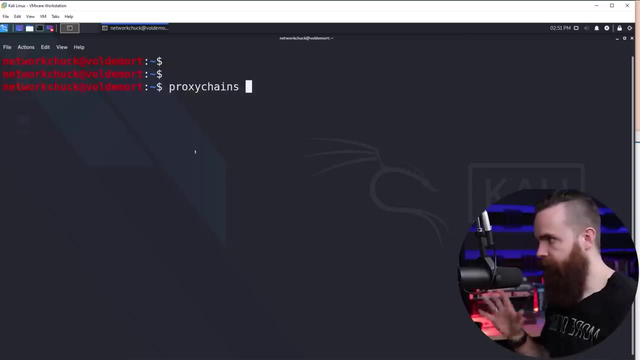 and the ports, and that's pretty much it. i'm going to hit escape colon wq to write and quit. done So now how do we use it? Watch this: I'll use a command: proxy chains. This is what you'll do whenever you want to use your proxies. You'll put this command right before. 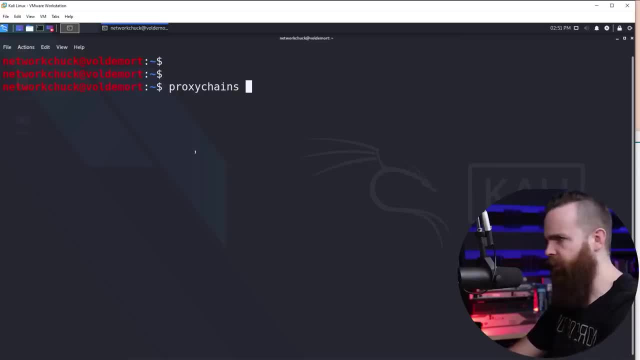 your other commands. So let's try out. um, let's try out Firefox. I want to verify this is actually working first, So I'll go out to googlecom and let's do it, And we're there now real quick. Let's go back to the command prompt and see what crazy stuff happened. And it's still happening. 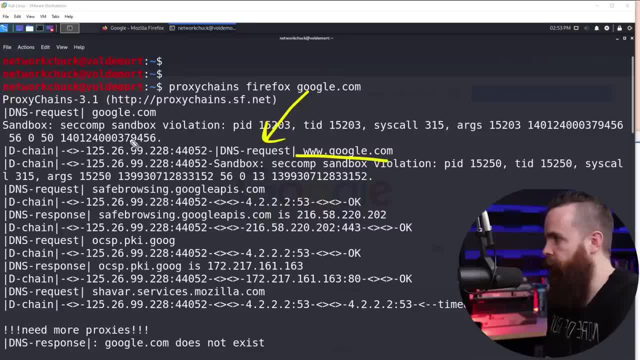 We can see here that first we have our DNS request to find out: Hey, where's googlecom? And we are indeed proxying it through that proxy I configured And once it learned the IP address of Google, it proxied our connection to Google through- well, the proxy. Now let's go see where. 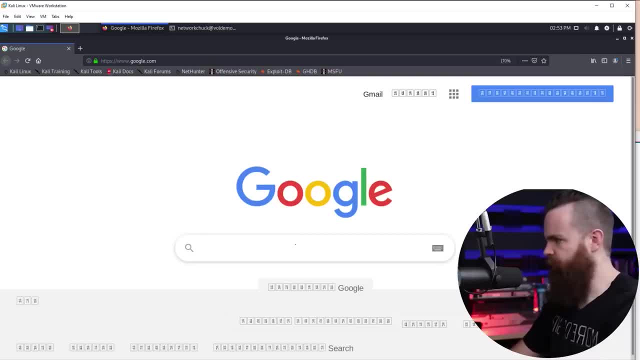 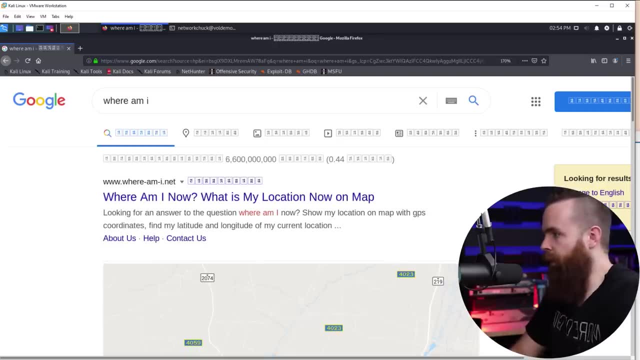 we are. Let me get back to our browser. I want to type in first. what's my IP address? So great? The public IP address does match up to the proxy I was using. If I type in, where am I? It's going. 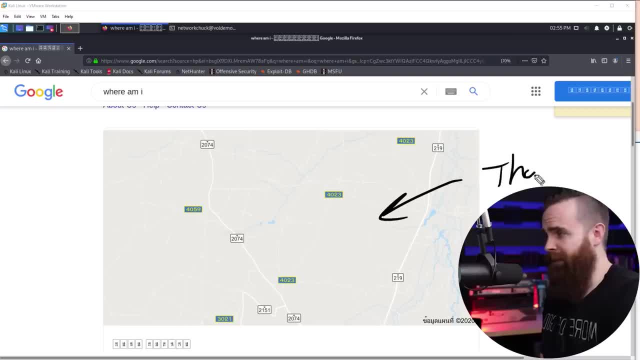 to tell me where I am, And this doesn't tell us much, but I can tell you right now that I am in Thailand, So good luck finding me. So I'm sending all of my commands through a proxy server in Thailand, which is: 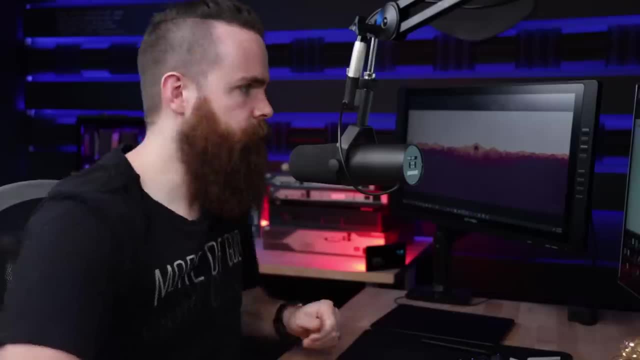 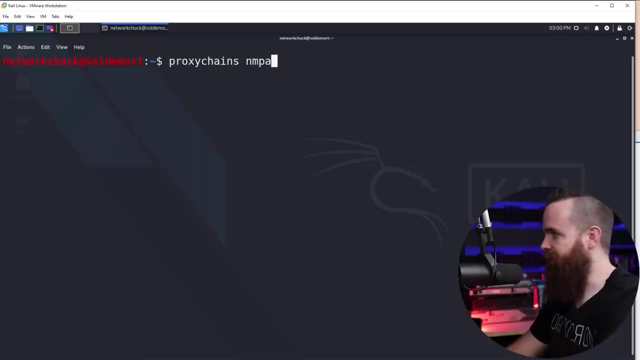 kind of crazy but also kind of cool. Like, let's try one real quick, Let's go back and hack David. David will never find me in Thailand. So once more, I'll start with proxy chains and I'll use the end map command. this time I'm going to use a TCP connect scan and I'll search for ports 80. 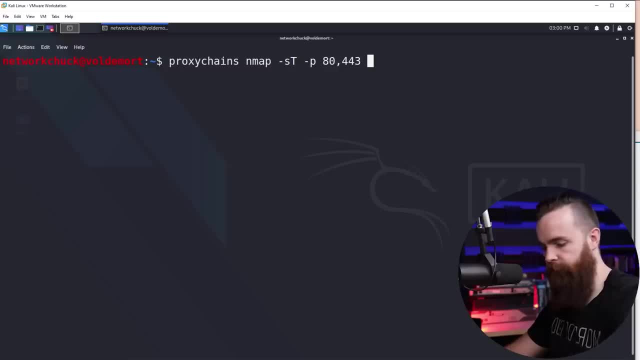 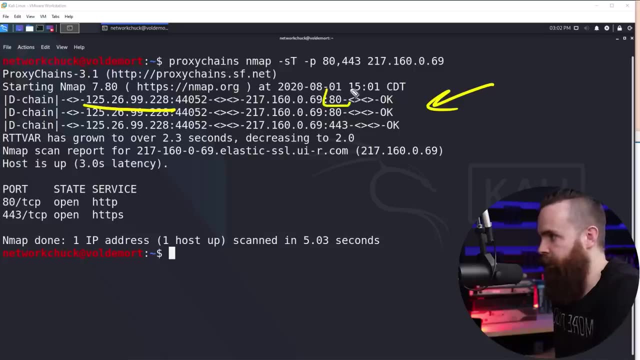 and 443 on David Bommel's website, And I'll use the IP address this time And let's see what happens Now. how cool is this? Every single command went through the proxy and went through Thailand to discover if these ports respond. So, as I'm pen testing David's site, as I'm doing, 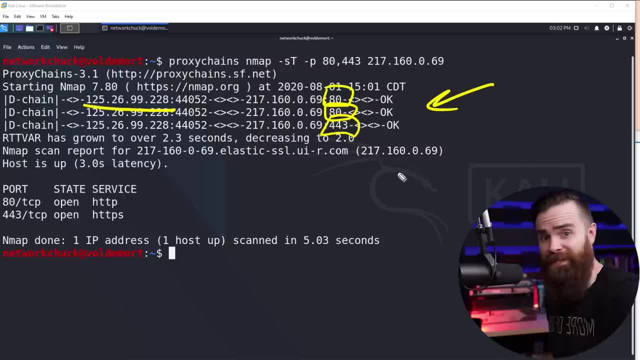 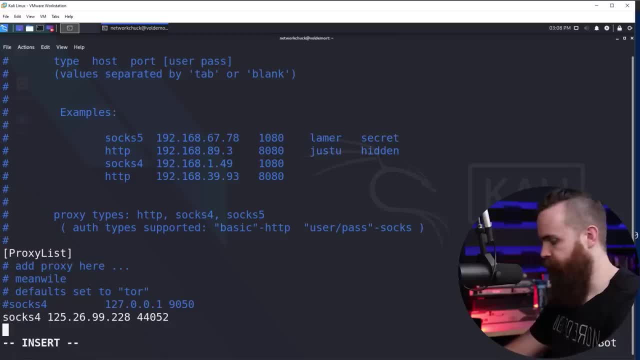 vulnerability scans and such. he doesn't know it's me, He thinks it's some person in Thailand and I get my info. Now, this is just one proxy. Let's add one more to the list. I'm going to hit I to start editing, and just below my 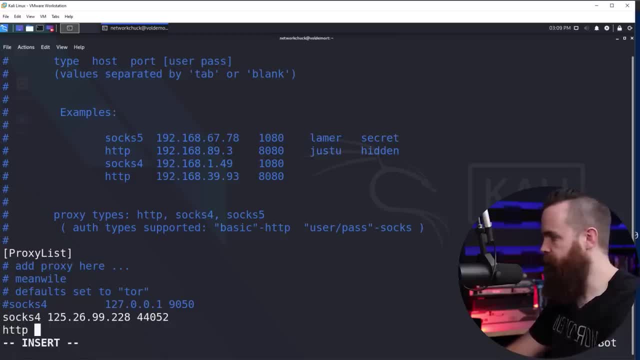 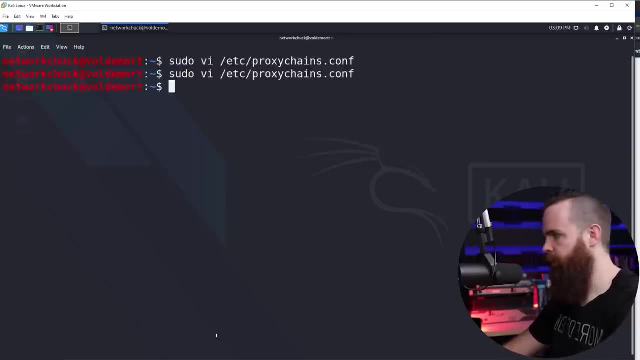 first server. I'll put my second server here. This one will be HTTP, and then I'll put a space and the IP address and then the port number- space 8888, escape colon, WQ- And we're ready to rock. Let's make sure it works. first I'll do proxy chains- Firefox, googlecom And, okay, looks like it may. 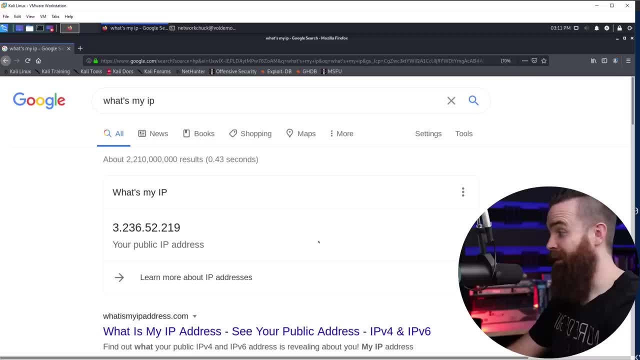 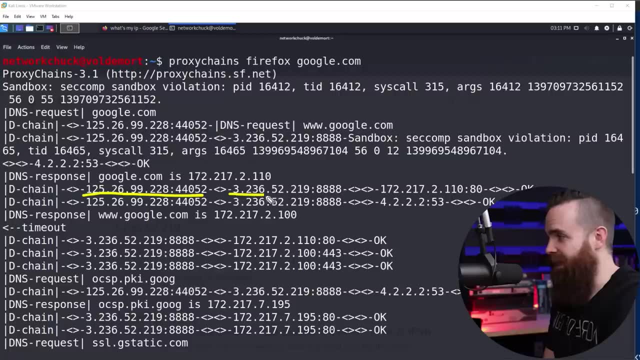 have worked. Let's do what's my IP And there we go, Look at that. Let's take a look at our command prompt. Here's the chain right here. How crazy is this? We first have our Thailand chain And this is actually a server on AWS that I 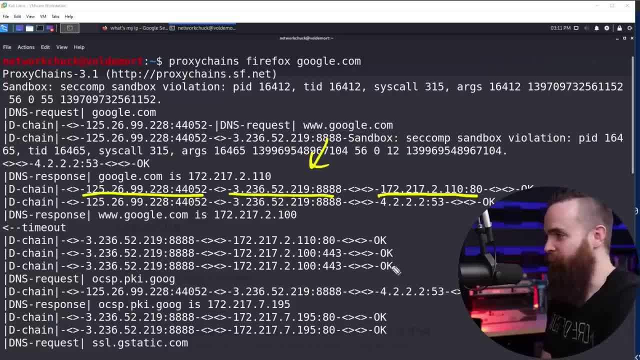 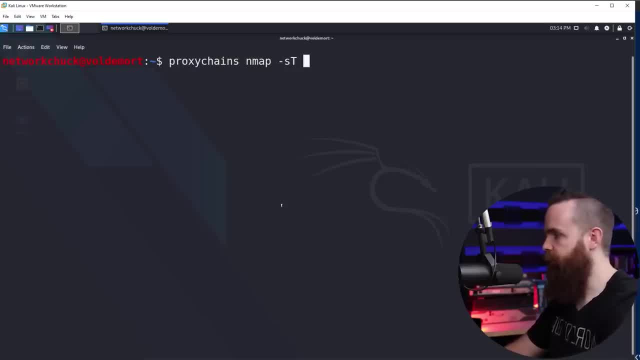 set up a proxy, I set up And then we're finally to Google. Isn't that amazing. I love that. Let's see how it looks when we use in map. So I'll do proxy chains and map dash st for a TCP connect. 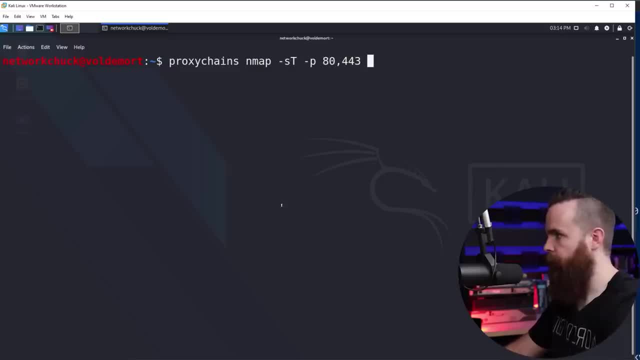 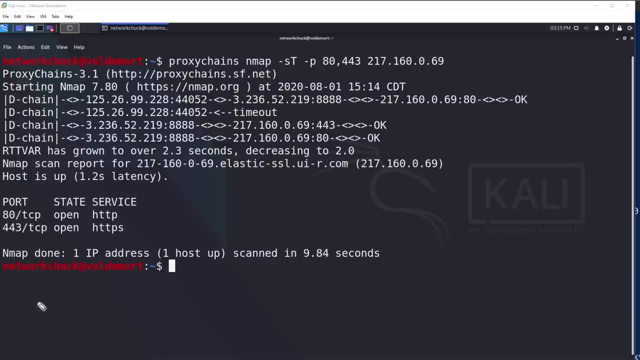 dash P and I'll put ports 80 and 443.. And then David Bommel's IP address. Boom, How cool is it. Look at this. It's going through the chain and checking. but how insane is this, It's going from. 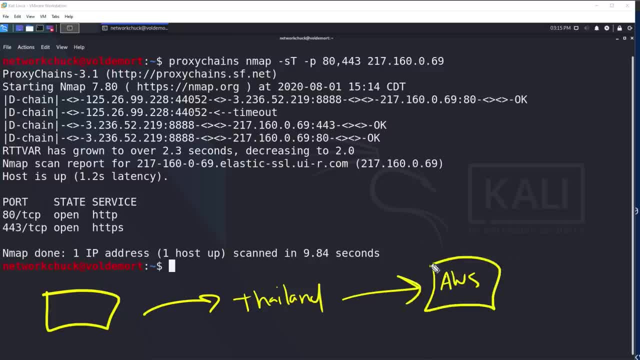 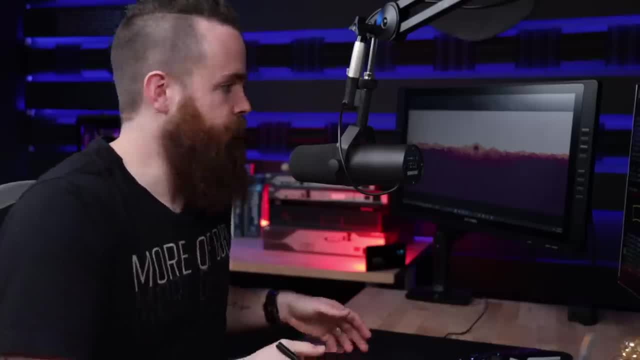 me to Thailand, to AWS, which I don't know where. that is specifically to David. How's he ever going to find me? And if I keep adding more proxies, I'm hidden man, I'm, I'm gone. Now I'm sure you're. 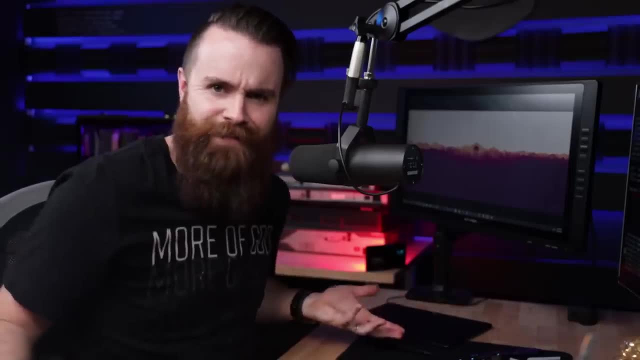 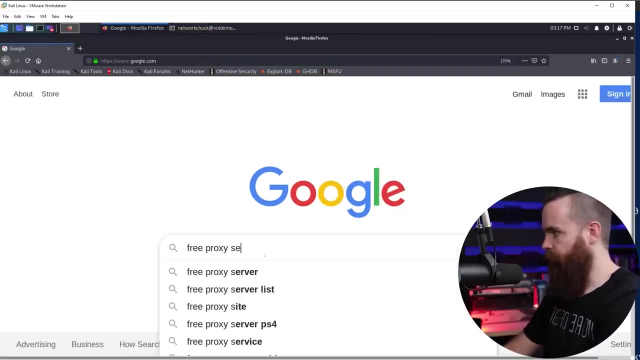 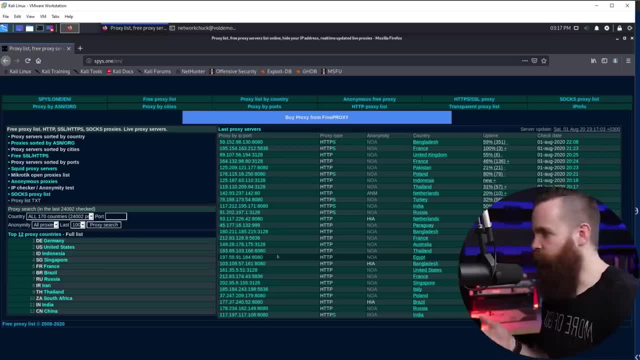 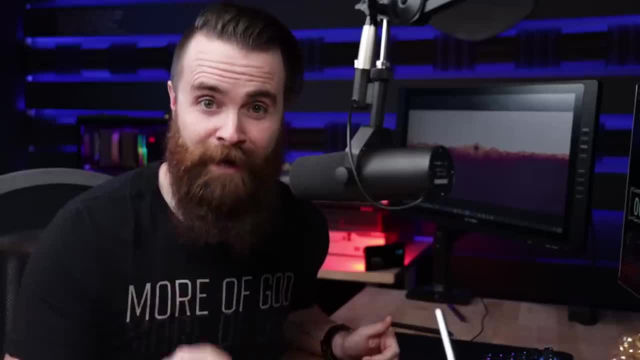 Now I'll tell you this: not all proxies are created equal or will work, So you might have to go through a few and test them, but that's how you would find them, just Googling and trying them out. All right, Are you ready for the challenge? Check this out. So this is the proxy chain challenge. Here's what. 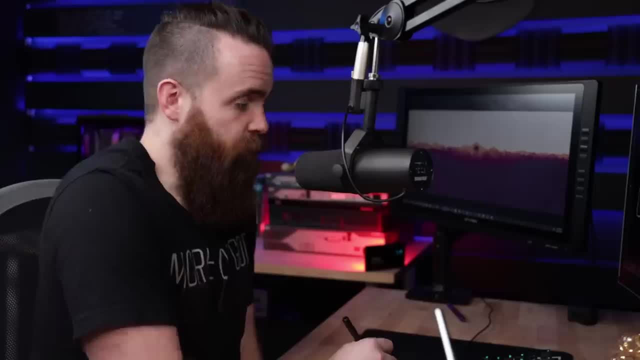 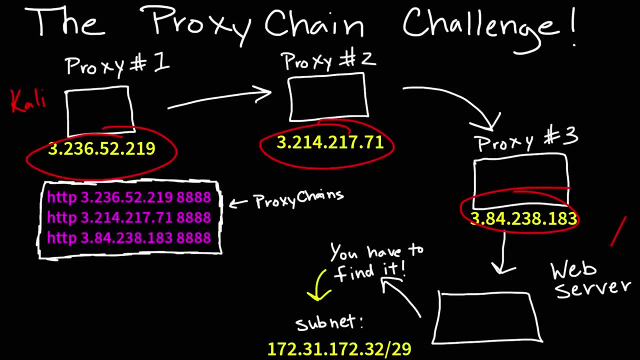 you have to do first. You will need Kali Linux to run this. You'll do exactly what we demoed in the video today, And the challenge here is that you have to use all three of these proxies to get to this web server right here, And this is. 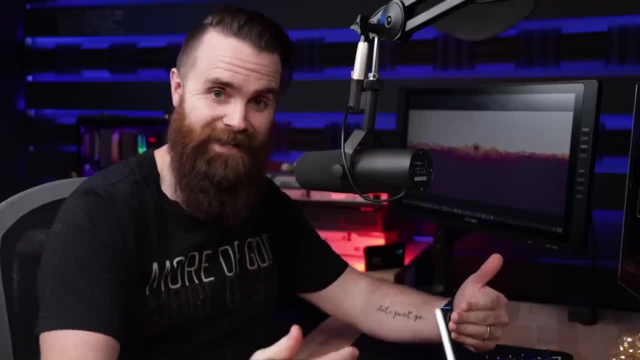 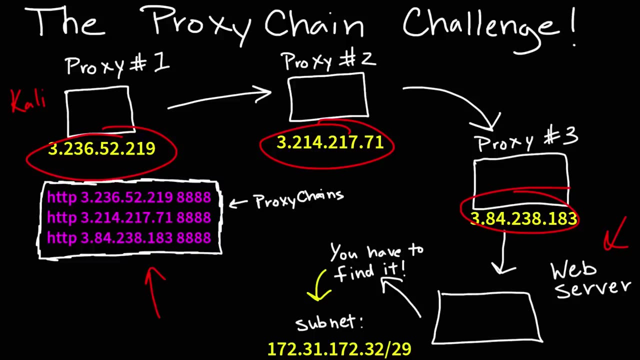 another. use the proxies. You can use them to hide yourself. You can also use them to gain access into other networks, which is what's happening here. Now you must use all three proxies in this order in your configuration file. Why? Well, because you can't access this proxy directly. right here You can. 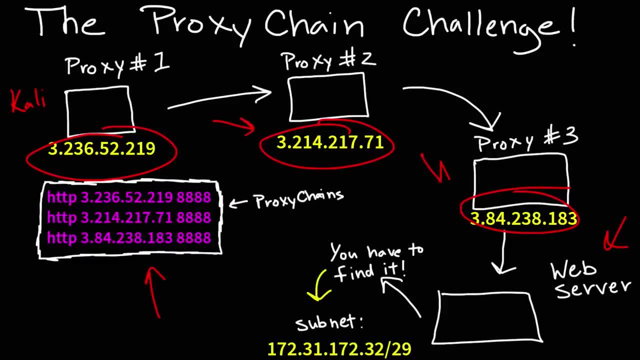 only access it from this IP address. You can't access this proxy directly. You can only access it from this IP address. So once you have your proxy set up and you have all your traffic going through these proxies, you'll get to here where you have to find this web server. 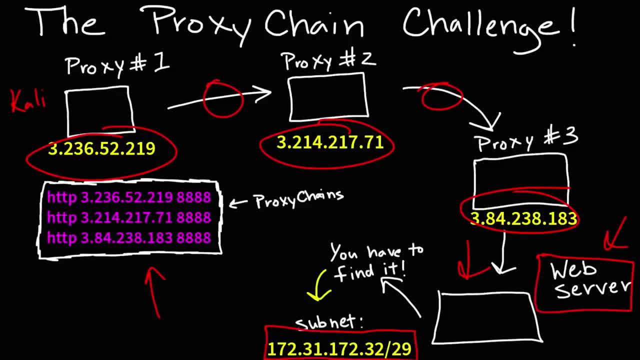 This web server has a private IP address And this range right here. The only way you can access these private IP addresses is by going through all three of these proxies. You'll need to scan this subnet using Nmap to find the right host that has. 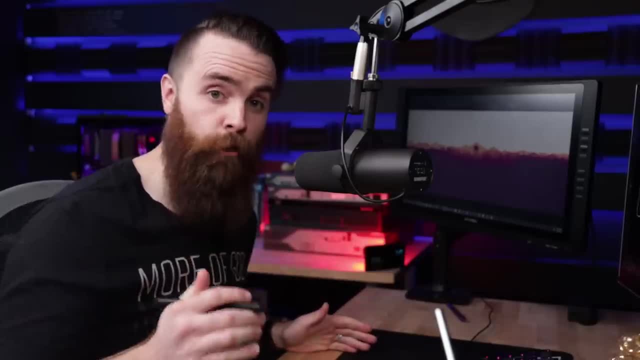 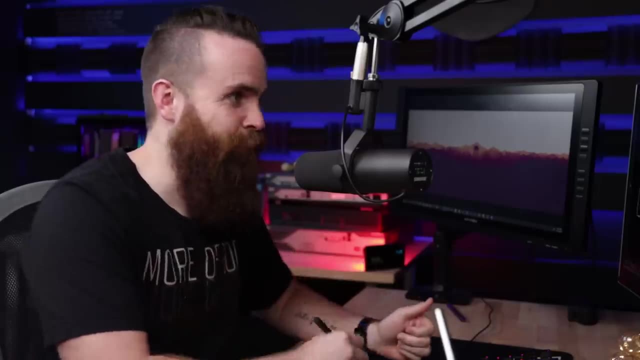 port 80 open. Once you've identified which host has port 80 open, then you'll need to access the website And, of course, you'll have to access it via the proxy chain. It's a private IP address that's only accessible through the entire chain, And on that website you'll have further instructions. 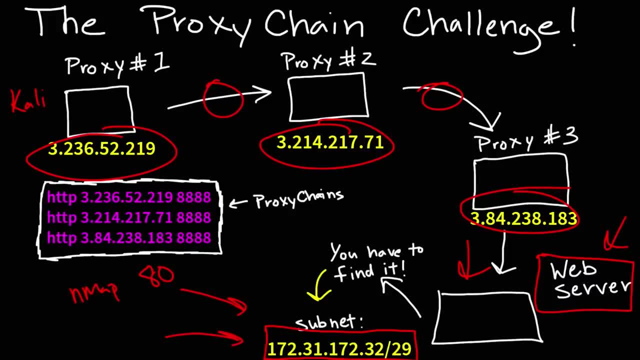 Now a hint on the Nmap stuff right here. None of the hosts in this group will respond to a ping And you may recall from the Nmap video that Nmap will initially send a ping to make sure the hosts are up before attempting to see which ports are open. So you'll need to make sure that Nmap isn't going to ping. 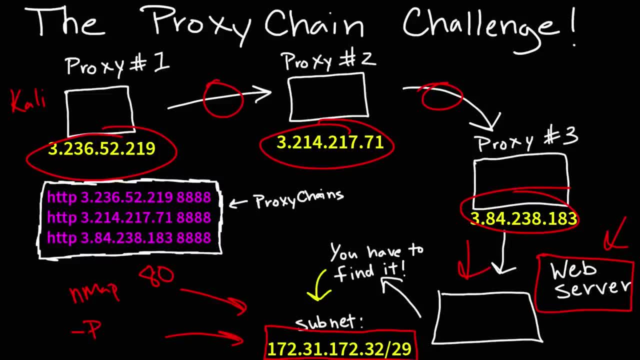 and do that check. To avoid that, we'll use the switch- uppercase P, lowercase N. This will avoid the ping, the initial ping, to see if the host is up, and just go for the TCP connect. And that's what I would do. I would use the TCP connect dash S, T, lowercase S, capital T And, of course, 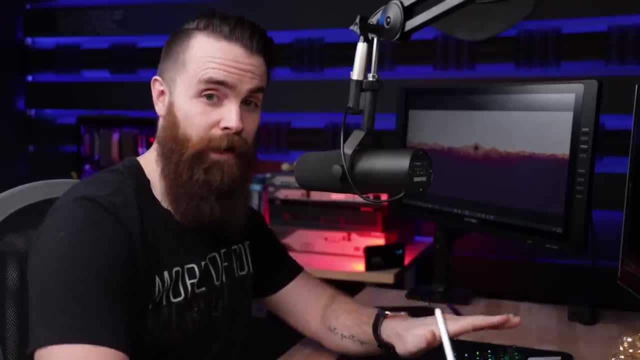 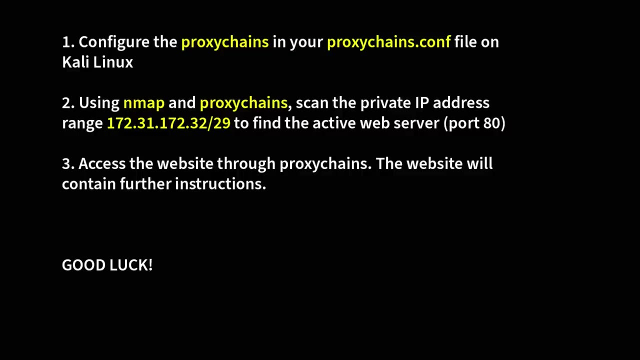 you got to use your proxy chains, Otherwise you'll get nothing. Okay, To sum this up real quick, you're going to configure the proxy chains I just showed you in your proxy chains file in Kali Linux. You'll then use Nmap and proxy chains to scan the private 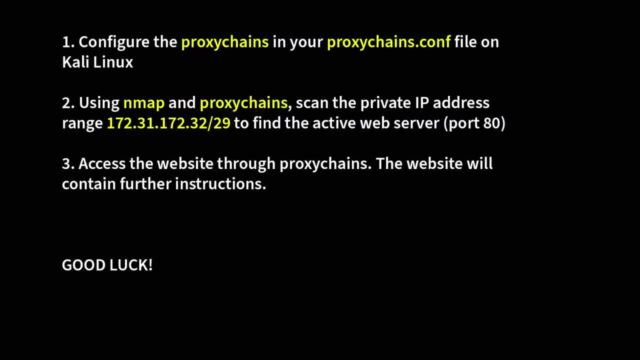 IP address range of 172.31.172.32 slash 29.. And you're looking for the active web server that has port 80 open. Once you identify which host that is, access that website through proxy chains And on that website you'll find the next step, the further instructions. Good luck, Only five.